and can motivate professionals to act in ways that violate their responsibilities and hurt their clients and employers. Doctors, for example, may face a conflict of interest when they are paid more for some procedures than for others. Their professional responsibility is to do what is best for the patient. 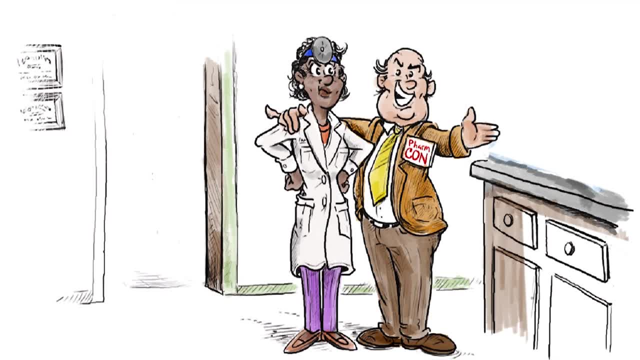 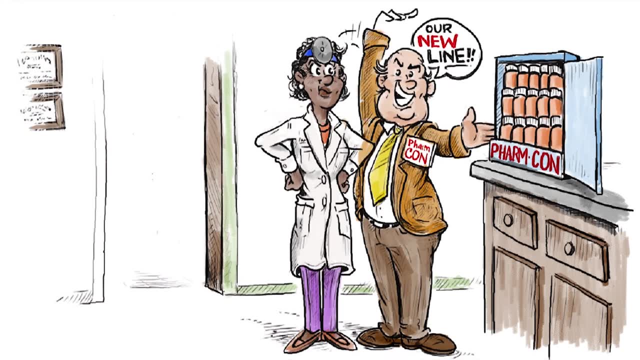 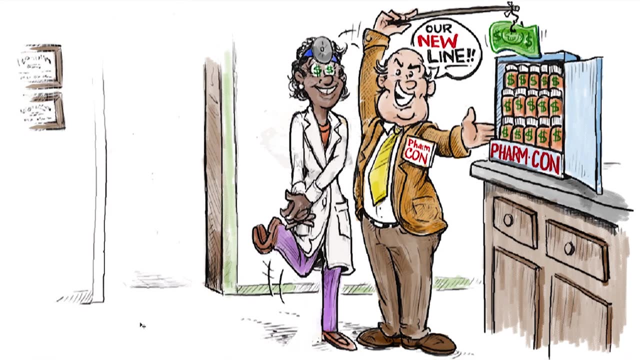 But their financial incentive is not always aligned with this responsibility. If an oncologist profits from selling chemotherapy agents to their patients, and some agents are more expensive than others, this conflict becomes a problem. Most doctors would never think of profiting in ways that hurt their patients. 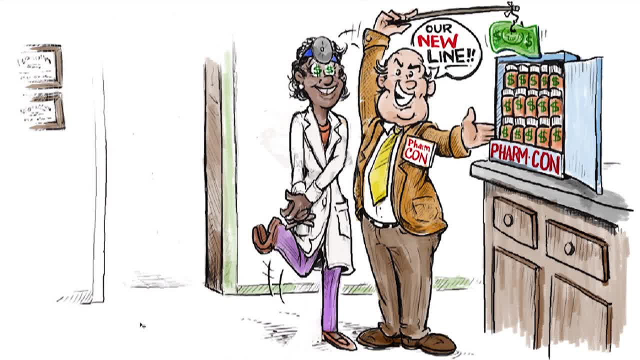 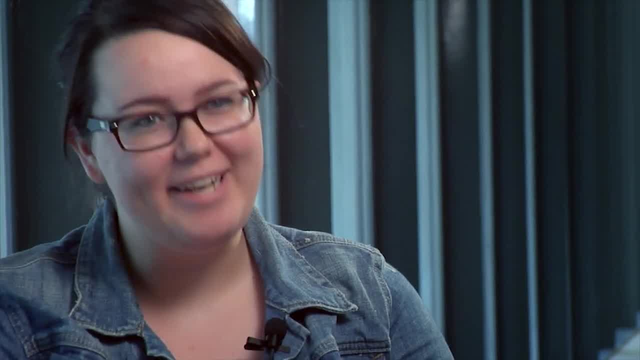 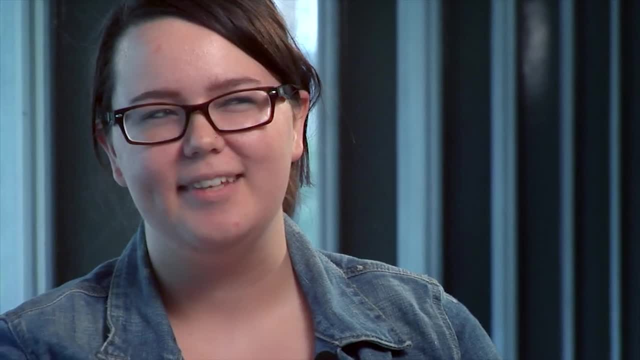 But some may either consciously or subconsciously. I run a magazine on campus and I start dating one of my writers and I'm the editor And he started getting entertainment stories that were not as good As the other entertainment writers And I was like: did I make that decision because he's improving in this section? 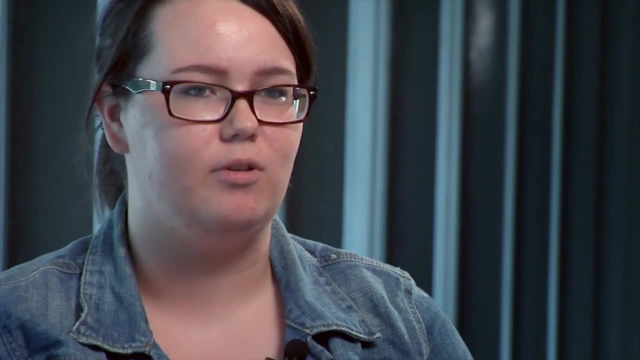 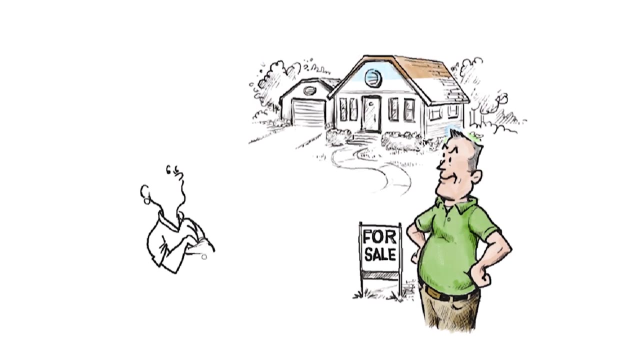 Or do I want to please him and make him happy on the staff as well as in our relationship? When there are conflicts of interest, you can almost guarantee that they will sometimes lead to bad outcomes. Surprisingly, in many states, real estate agents can represent both the buyer and the seller in a home transaction. 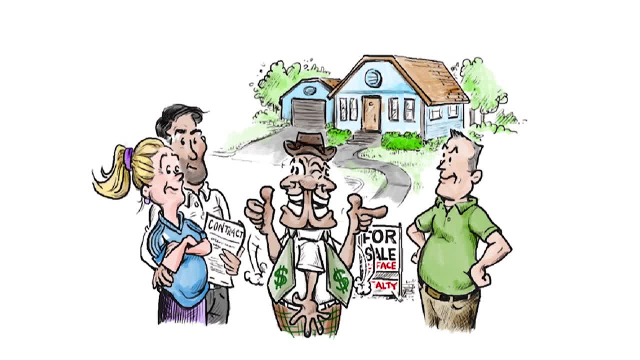 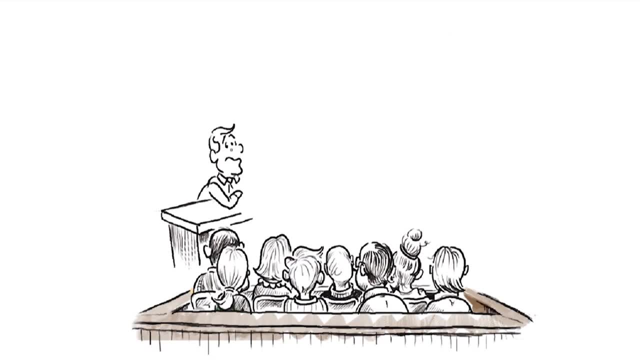 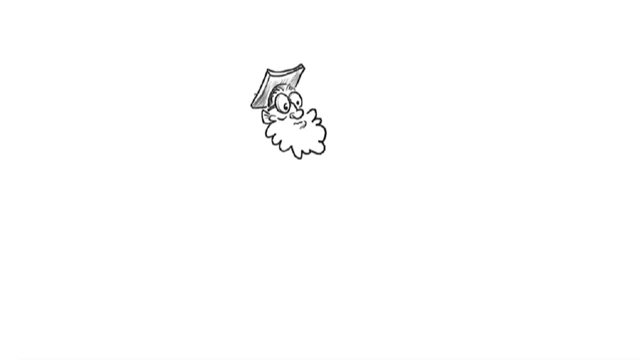 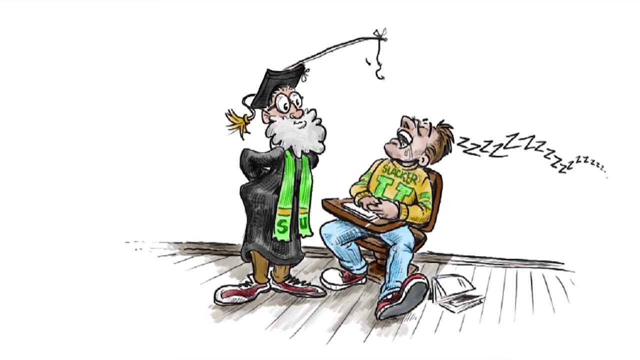 The conflict in such transactions is clear. An agent could never have both parties' best interests in mind, Just as an attorney could never adequately represent both a plaintiff and a defendant in civil lawsuit. Even professors face a conflict of interest when they're designing courses that will be evaluated by students seeking high grades and low workload. 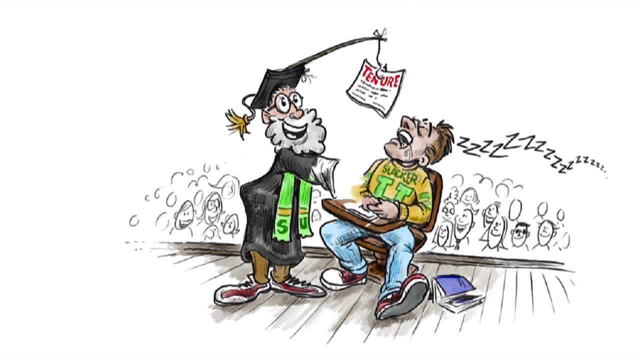 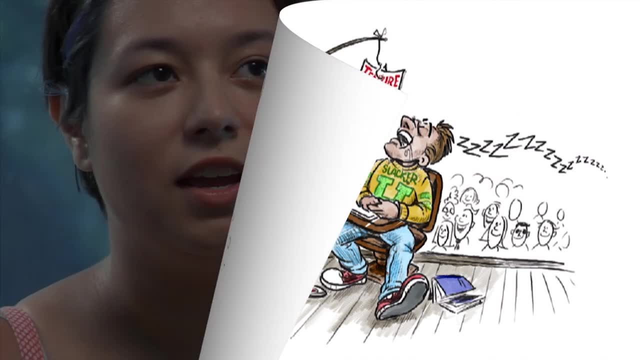 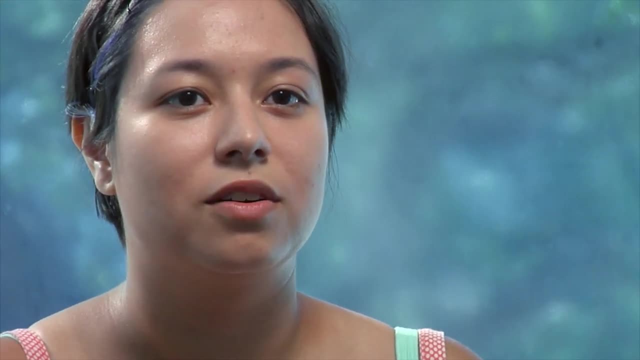 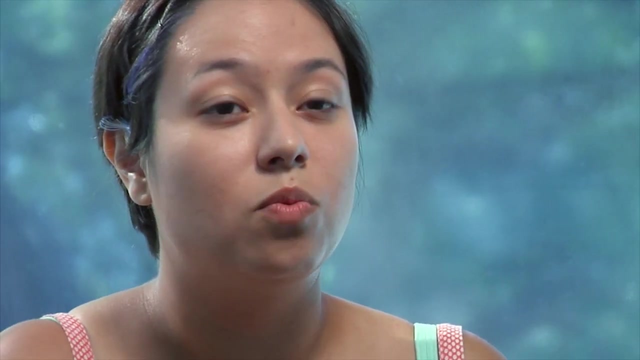 If the professor is ultimately promoted based on their popularity with students, will they consider making the course a little easier? If, every single time, someone got a lower score in a class than they expected and that counted against the professor, it doesn't really add up because you're not encouraging the teaching faculty to do what they are there to do. 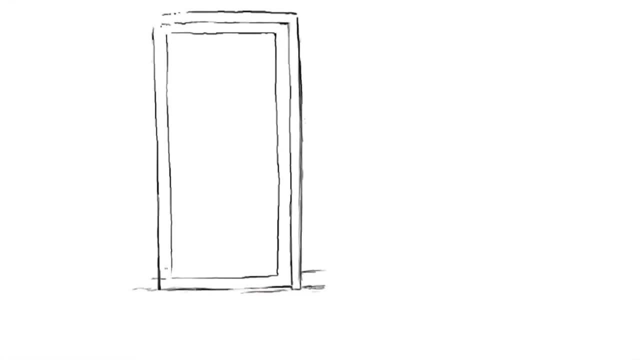 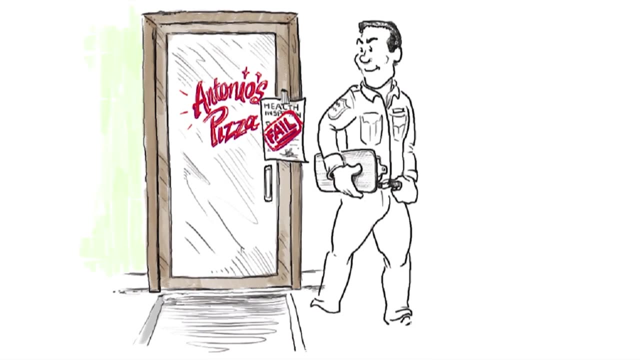 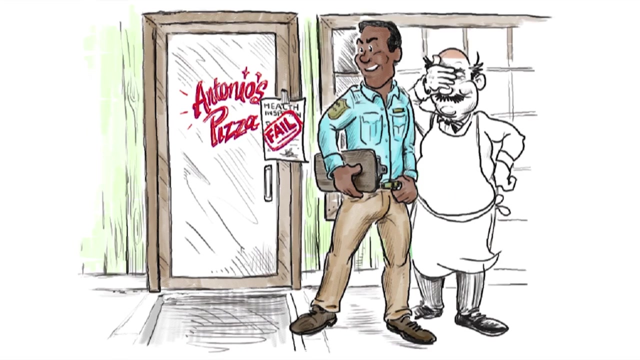 is to challenge students and push them. The key implication is that managers and policymakers must constantly evaluate whether professionals and employees might face incentives to act counter to their responsibility. Eliminating conflicts of interest is one of the simplest and most effective ways to reduce unethical behavior. 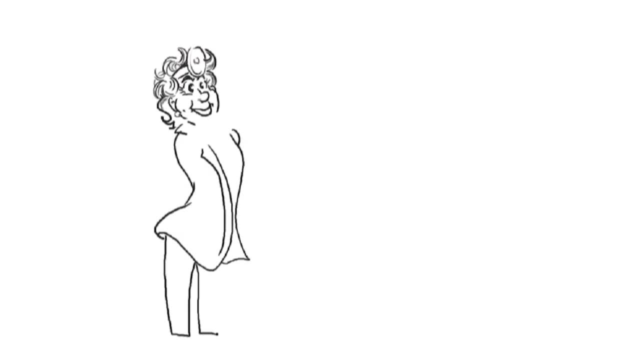 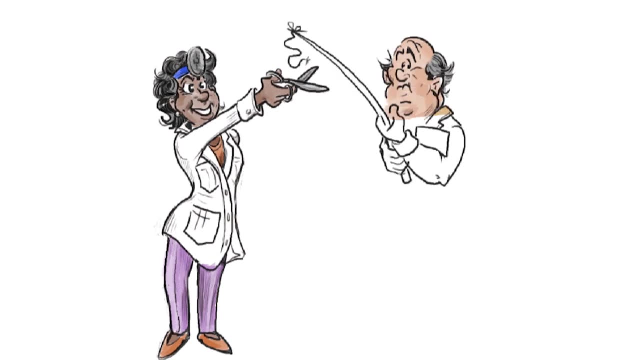 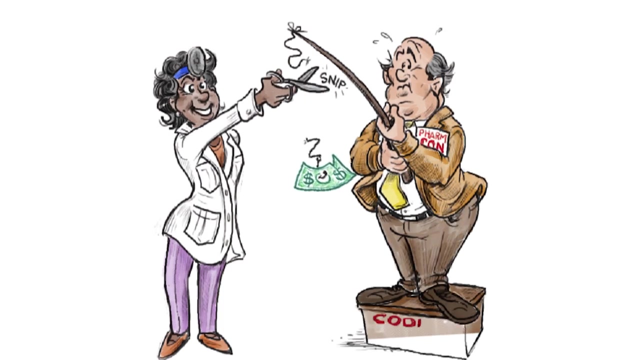 But in order to do so, we must be willing to acknowledge that professional codes of conduct, like those followed by doctors, lawyers, accountants and real estate agents, do not make people immune to these conflicts, And that these codes are rarely a justification for ignoring the likely outcomes that conflicts of interest create.